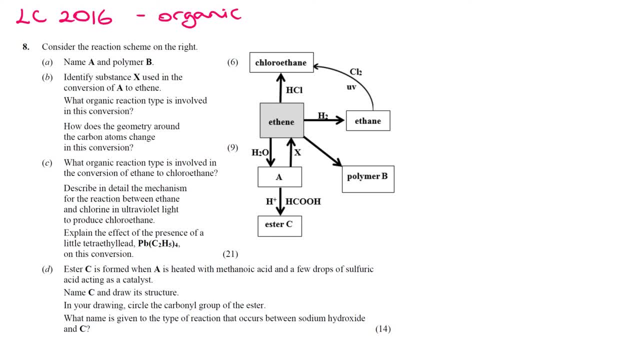 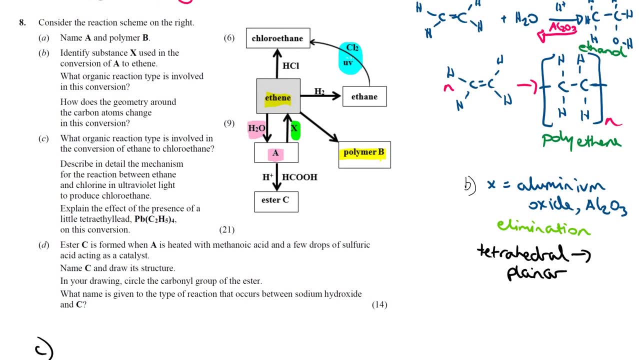 In this video I'm going to go through a Leave and Surpass paper question on organic chemistry. It's 2016,, question 8. I'm going from ethane to chloroethane. that's a substitution reaction, a free radical substitution. 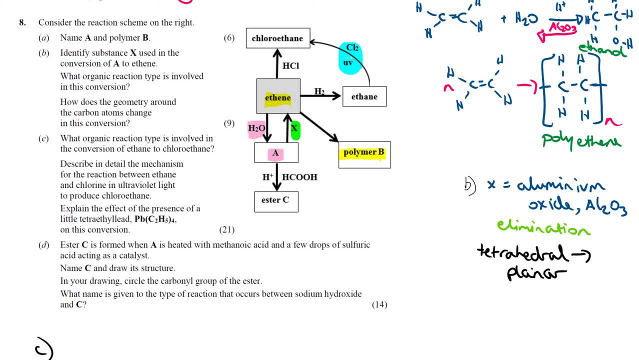 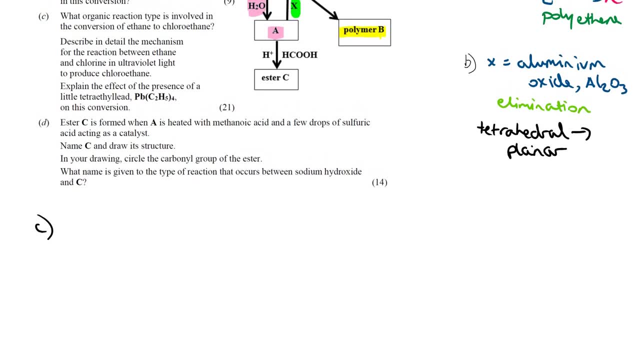 Describe in detail the mechanism for the reaction using UV light. Okay, so I'm going to go through that now. So the reaction that we're talking about is the reaction of ethane, which is C2H6,, and chlorine in the presence of UV light to form chloroethane. 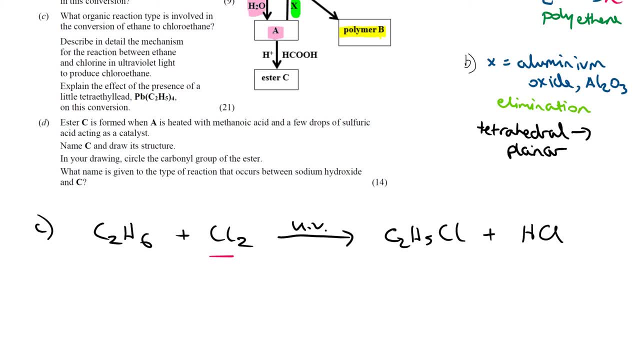 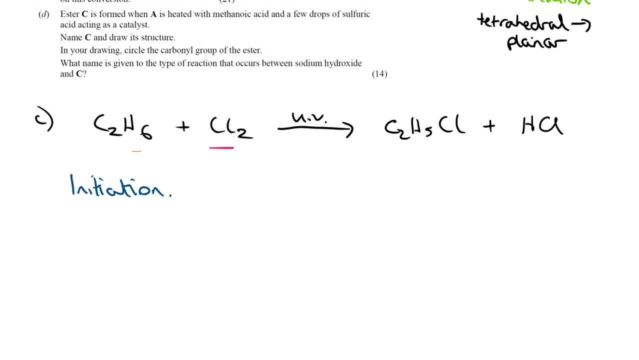 And substitution reaction, because we're substituting one of the chlorines there for one of the chlorines in the presence of UV light. Okay, So we have an initiation step to begin with, and this is where the UV light homolytically breaks apart the chlorine molecule. 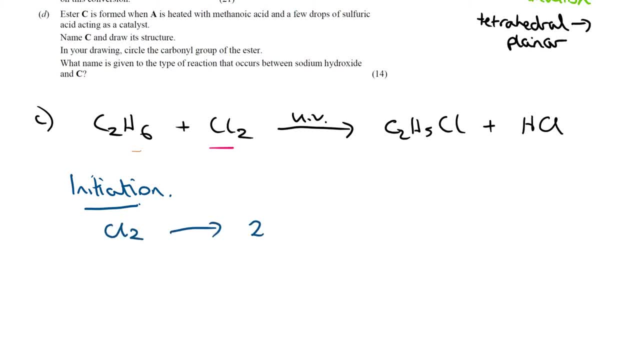 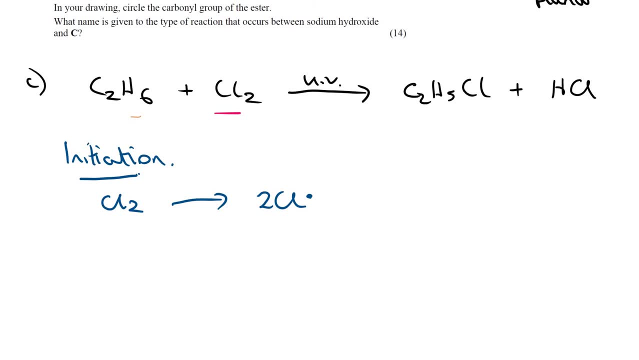 So Cl2 just breaks into two chlorine radicals And I'm just going to draw my radical with a dot. So just going to describe on the side here what happens: You've got a chlorine molecule And I'm just going to draw my radical with a dot. 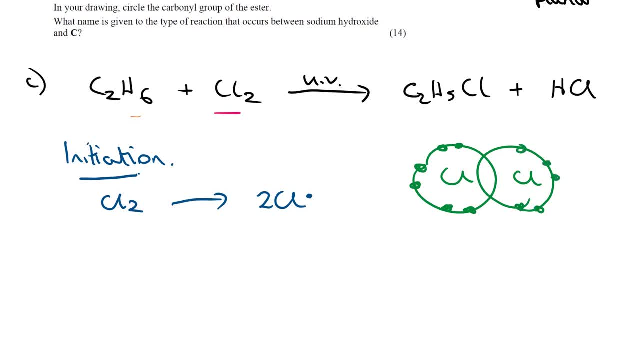 So I'm going to draw the dot and cross diagram for each of the chlorine atoms. when they're covalently bonded, Okay, And all that happens? the UV light breaks apart the shared pair and each of the electrons just goes straight back onto the chlorine atoms. 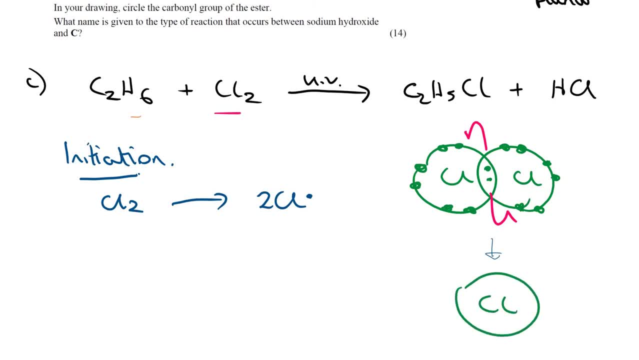 So you're left with two chlorine atoms in their original state. Of course, these are not very stable. That's why chlorine exists as a diatomic molecule. Okay, Okay, So you form two of them Now. free radicals themselves are quite reactive. 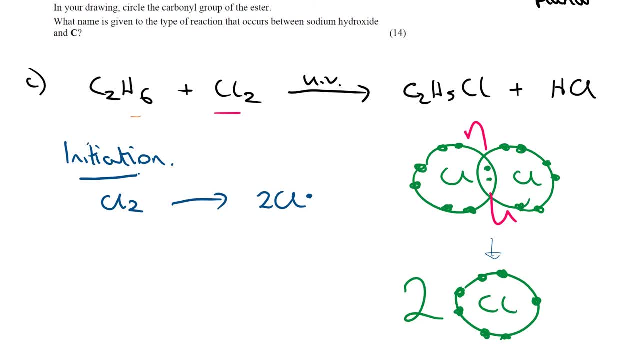 So what they can do is they can react with other molecules And in many ways its chemistry is hard to control. But that's just showing you what is happening. in each step The UV light breaks apart the shared electron pair and you form two chlorine atoms. 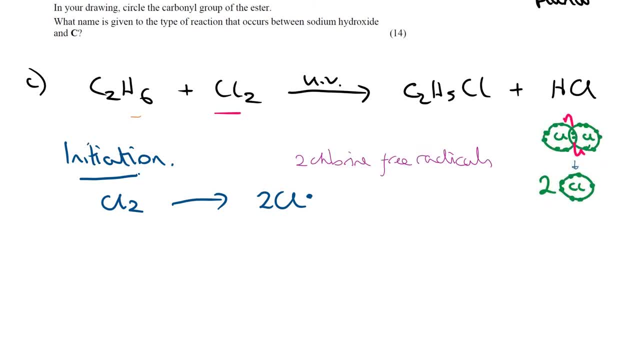 And we're going to call them free radicals, So I'm just going to put that to the side. So the next step is called propagation, And that's where our free radical is going to go and do something there. So we form the chlorine free radical here. 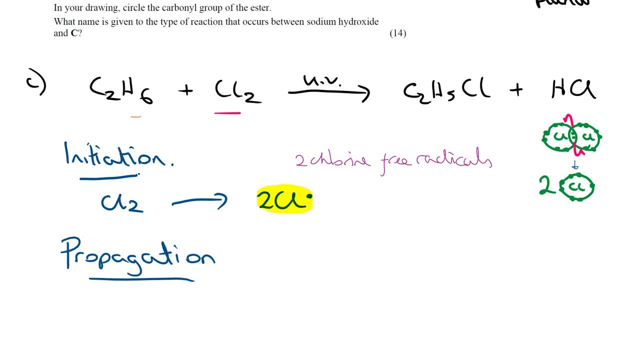 Two of them in fact, And the first propagation step is where one of the free radicals will react with the other reactant in the chemical equation. So that was our ethane C2H6. And all it does is- and I've described this in detail on the website- 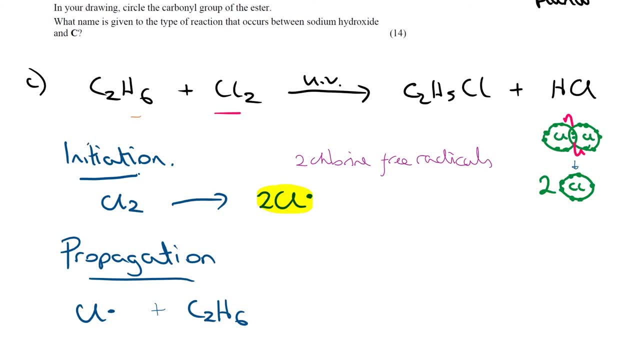 all it does is the free radical will abstract a hydrogen atom and you will get another homolytic breaking of the hydrogen atom and its carbon atom's covalent bond, where you get even breaking of the electrons, And so you form a carbon radical. 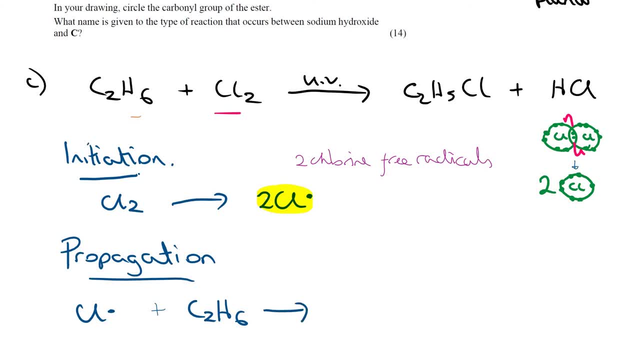 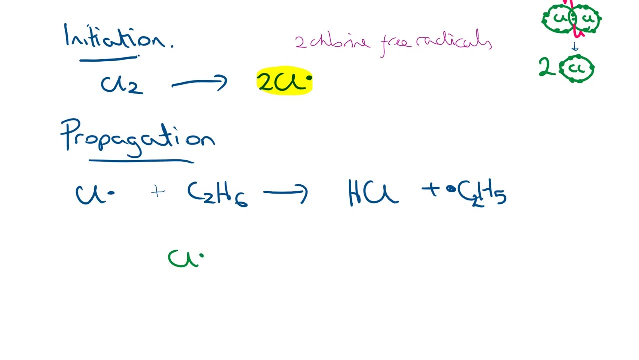 So they react and it just takes a hydrogen atom away. So you form HCl With a radical on the carbon. So just to explain that in a little bit more detail here: the chlorine radical sees the ethane And what happens is: 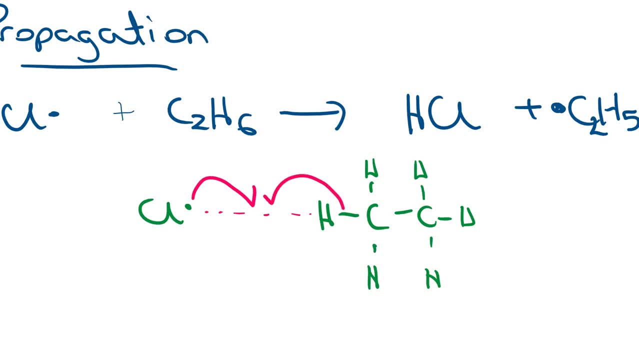 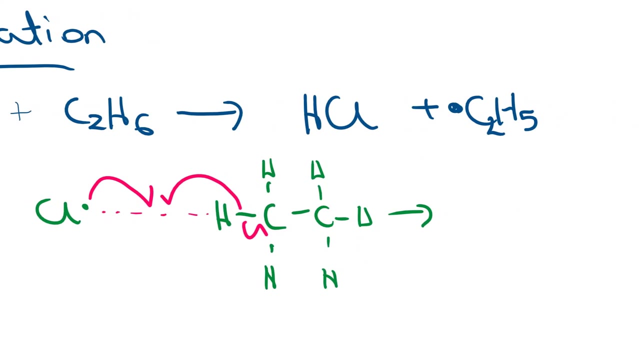 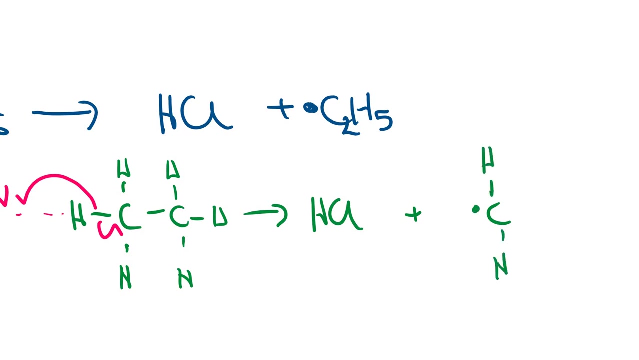 that electron and the hydrogen electron come together and form a shared pair of electrons. So we form hydrogen chloride, the molecule, And then this electron gets broken off and forms onto the ethane. You're left with HCl and this radical There. 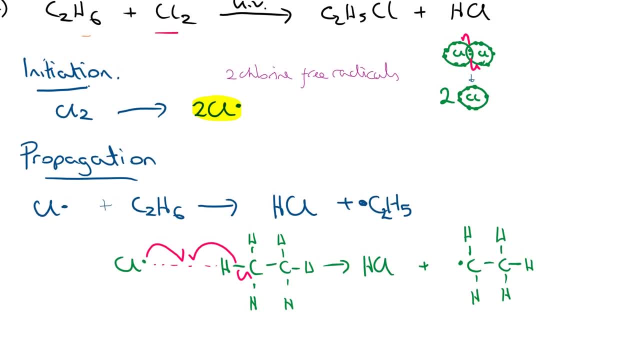 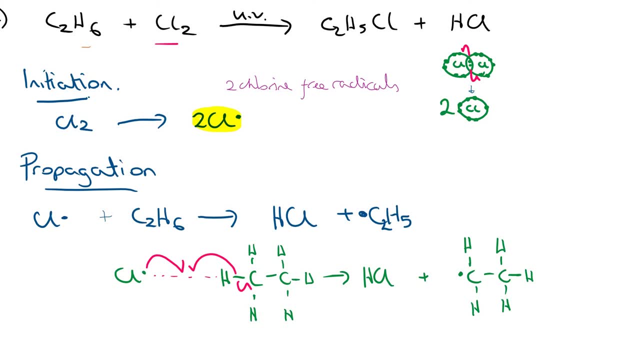 Now we've formed a different radical And the HCl is a molecule which won't react again here. But this other radical that you formed, as it's a radical, you've got a carbon with a single electron on it, so it's quite reactive. 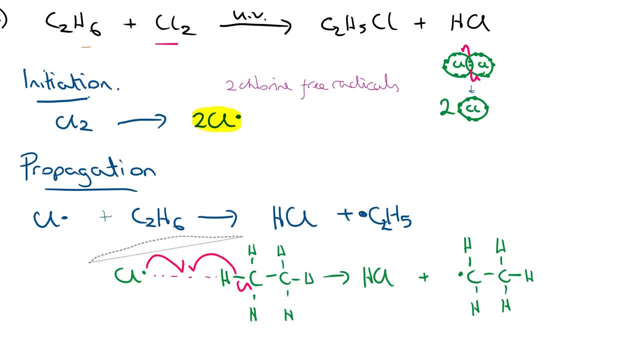 That will go and react with something else. So that's what's going to happen next. So there's a second propagation step whereby that radical that you made, C2H5, and I'm just drawing the radical on a carbon. 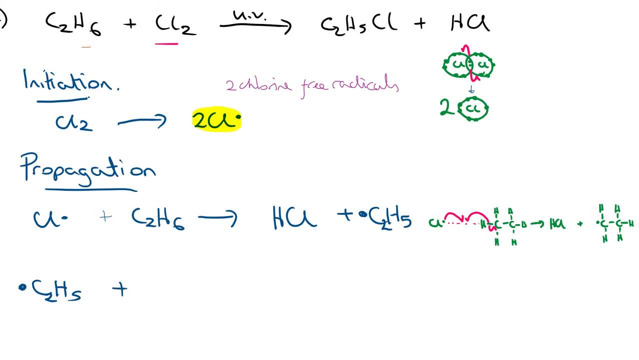 because that's where it actually is- reacts with the other reactant, which is chlorine molecules. Okay, And as that reacts, we form this radical, just forms a chemical bond with one of the chlorines And you form C2H5Cl. 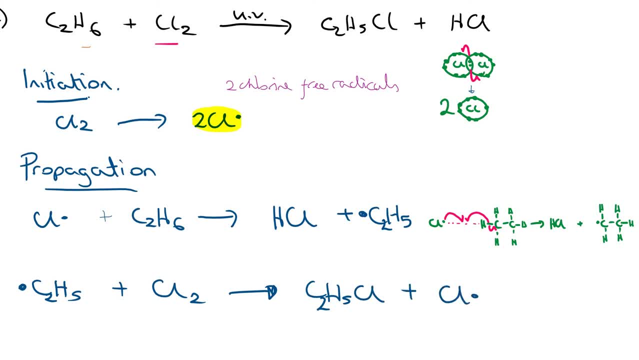 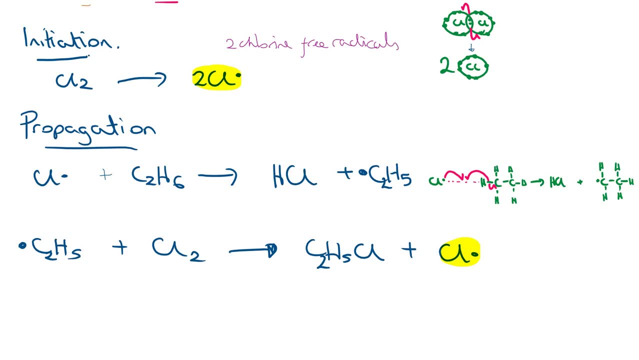 which is our desired product, And we reform our chlorine radical there, our reactive species. So again, just to show you how that happens: you've got CHH H, C H H with a radical And you've got chlorine. 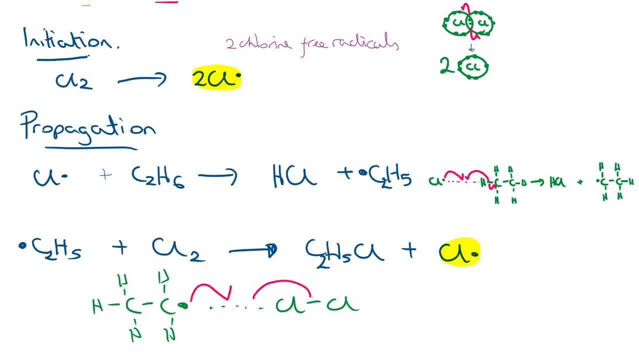 And what's going to happen here is that and that are going to. So a single-headed arrow, I should have said at the start- That shows the movement of one electron. So what you have here is you have this product, which is the one you want. 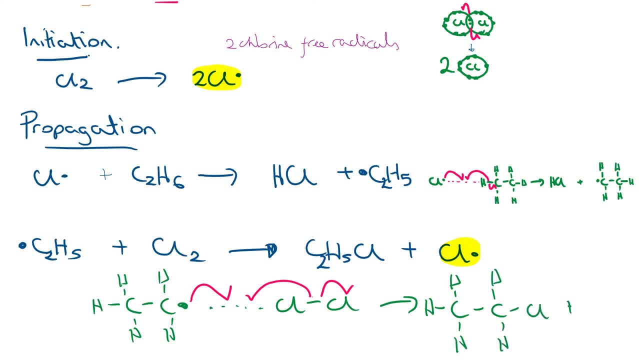 And you have reformed a chlorine Right Radical. Okay, So we've formed the desired product here. So normally, once you form the desired product in the mechanism you're going to finish. But because this is radical chemistry, 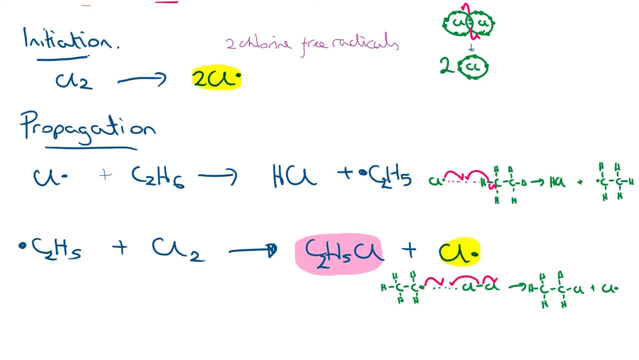 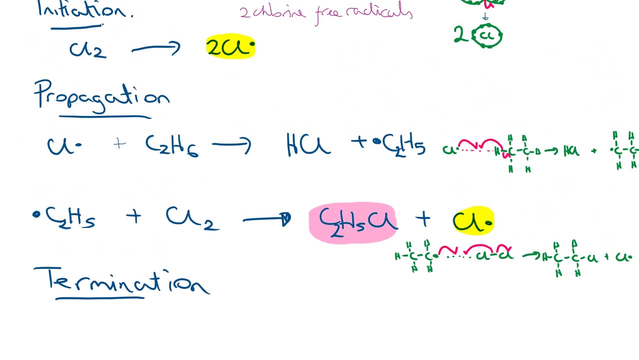 there's a lot of stuff that's still there that needs to be killed off, essentially. So we have these termination steps, which are basically steps that allow us to finish the reaction by not having any more radicals In the termination steps. all that's going to happen is 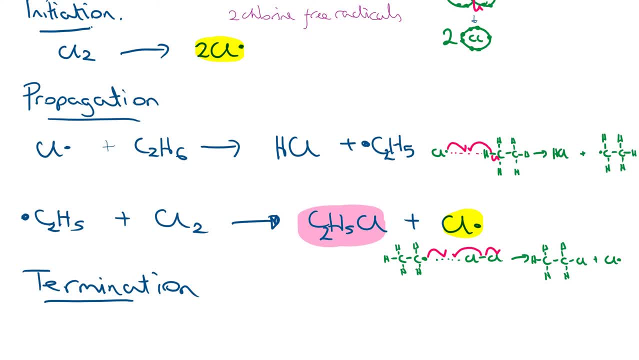 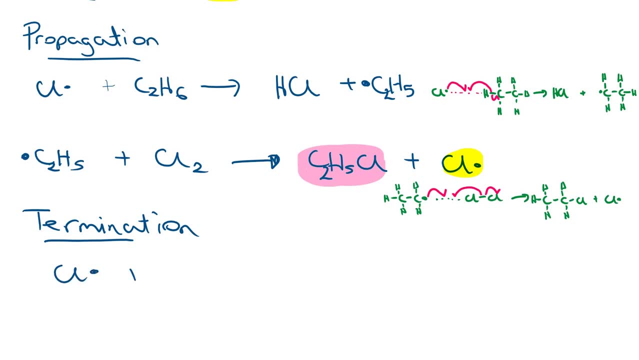 our free radicals are going to react with themselves and you're going to be left with neutral molecules. So the first one will be our chlorine- you could say Chlorine radical could react with a chlorine radical In the reverse of our initiation step. 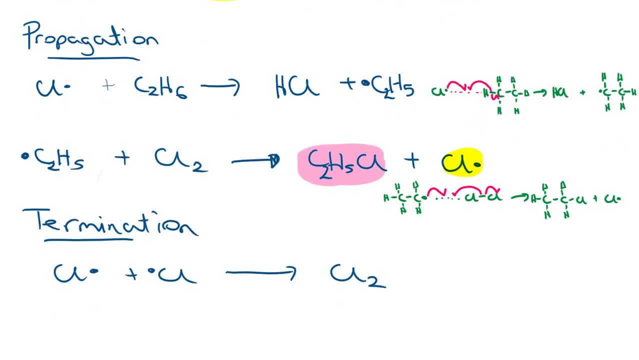 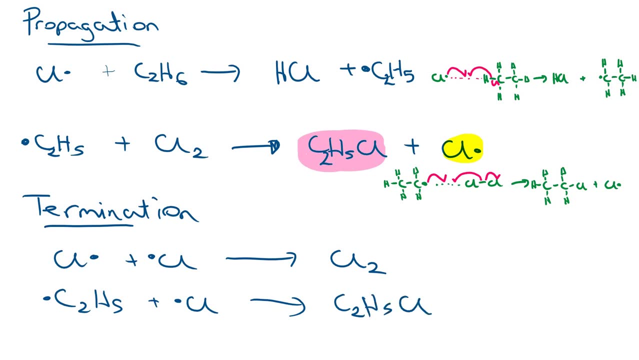 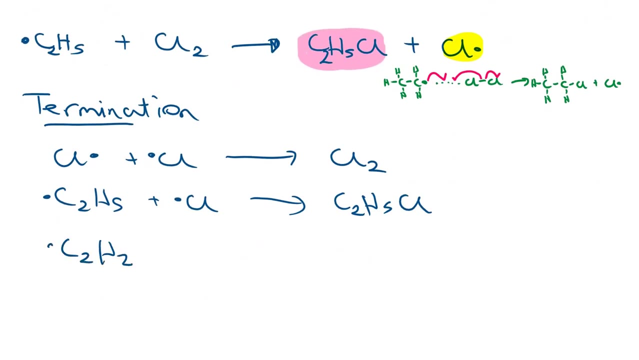 to form a chlorine molecule. we could have an ethyl radical and a chlorine radical Reacting to form the desired product there And lastly, you could actually have two ethyl radicals coming together. You've got an ethyl radical reacting with another ethyl radical. 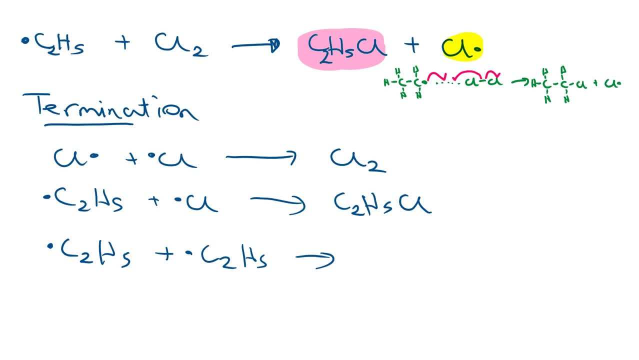 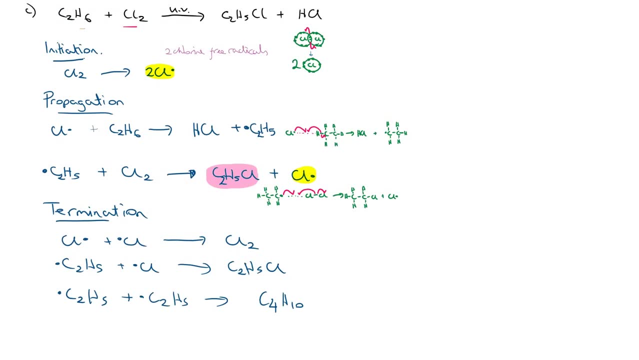 And what happens here is you do. when these two radicals combine, you get C4H10, which is butane. So this is our mechanism. All you need to remember are the steps in blue there, So it's important to try and remember them all.